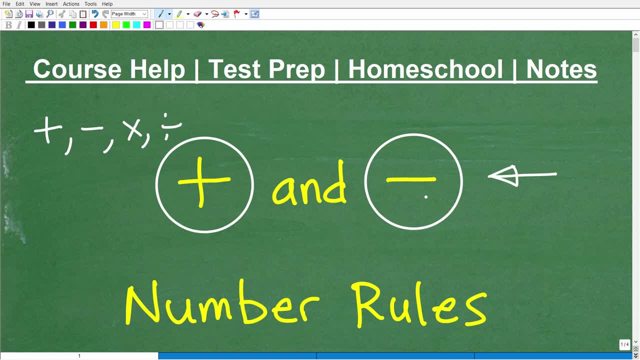 test or quiz back and you have errors in there. So you're not alone. but tell me if that's been your experience and you're like I need to figure this out once and for all. But anyways, I'm going to help you figure this out And I've done other videos on positive and negative number rules. 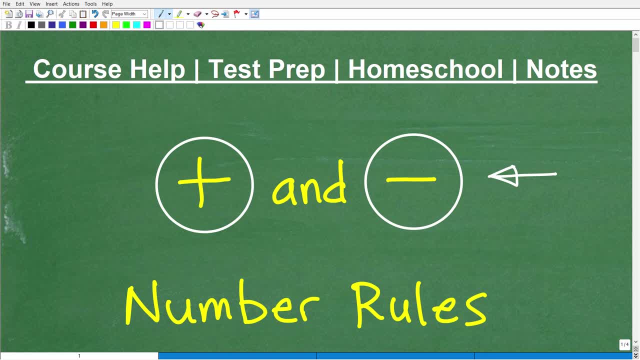 before in the past, but this is just a good topic to continue to revisit so we can be successful in mathematics. But before we get going, let me quickly introduce myself. My name is John. I'm the founder of Tablet Class Math. I'm also a middle and high school math. 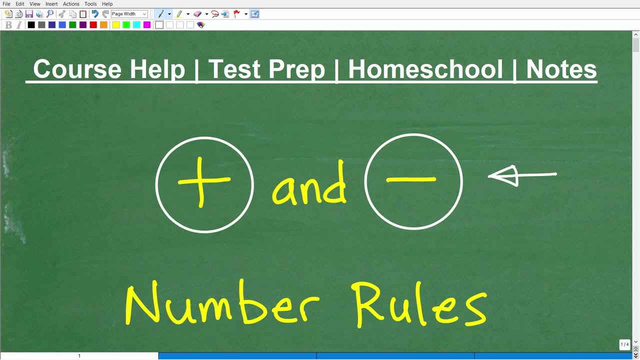 teacher And if you've been struggling in math, okay. if you just feel like you're not getting the right amount of instruction, or you just need more support than you're able to get from your teacher, or whatever the case might be, or if you want to get ahead, then you definitely got to check out. 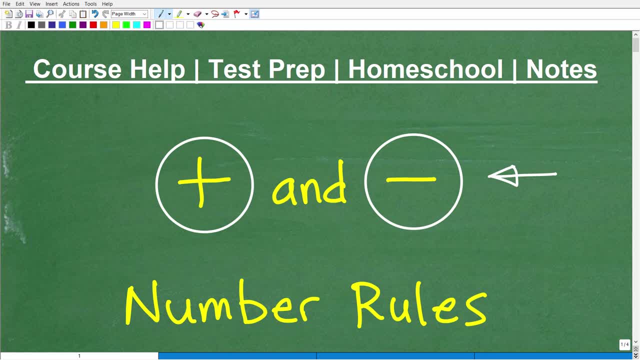 my math help program. Again, I'm going to leave the link in the description of this video, But my focus is for those of you that are in middle school, high school, even college level mathematics. So if you are struggling in math or if you want to get ahead in math and really want, 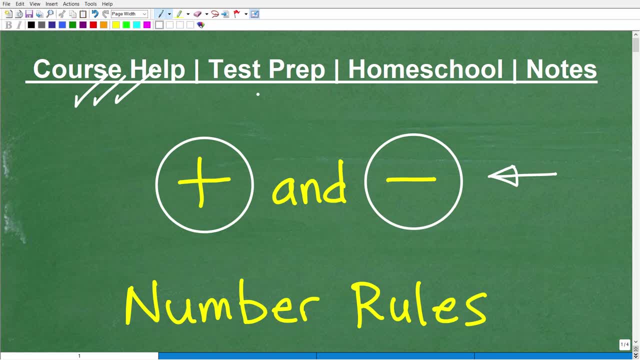 to lock in a great grade. I can definitely help you out Now if you are studying for any test that has math on it. so I'm talking about things like the GED, SAT, ACT, GRE, GMAT, ASVAB, ACCUPLACER. 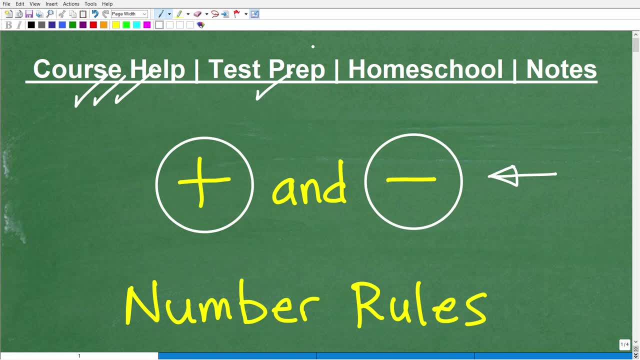 ALEC exam, CLEP exam, teacher certification exam, nursing school entrance exam. I can go on and on and on. There's so many different exams out there that have math on it. I can help you prepare and pass those exams. If you homeschool, you absolutely must check out the Tablet Class Math. 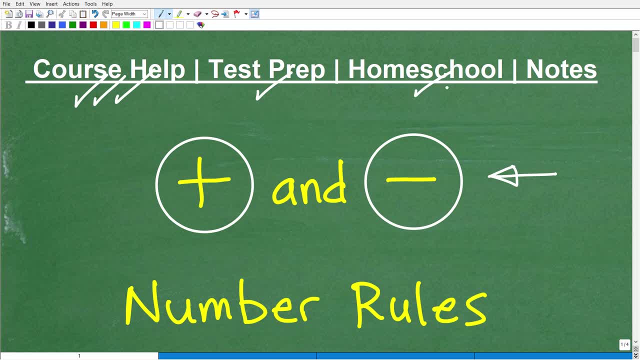 Program. Check out my homeschool math curriculum and program. I've been very successful working with homeschoolers for many, many years And if you don't have any math notes, don't panic, You can use mine. I'm going to leave links to my math notes in the description of this video, But if you 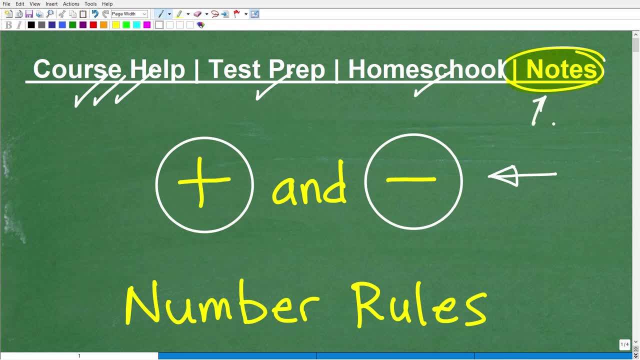 want to be great in math, and if you want to have great grades in mathematics, you got to take great math notes. Just trust me on this. There's no getting around taking awesome notes if you want to do awesome in math. Okay, so let's get going here. Quick power review. 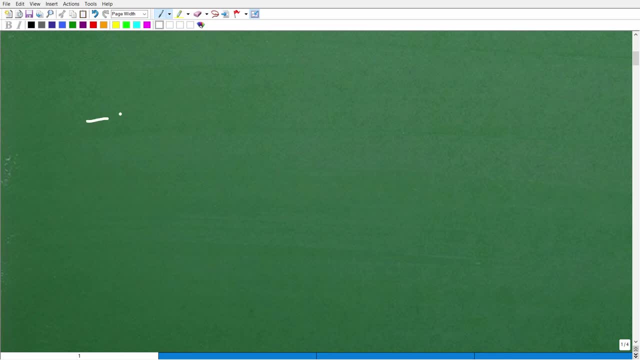 On positive and negative numbers. So we're talking about problems like this: Negative 7 plus 8, or negative 3 times negative 2 or negative 16 divided by 4, or negative of a negative 5.. These are the type of problems we're talking about. Or let's do another one: 1 minus 9.. Okay, so this is what. 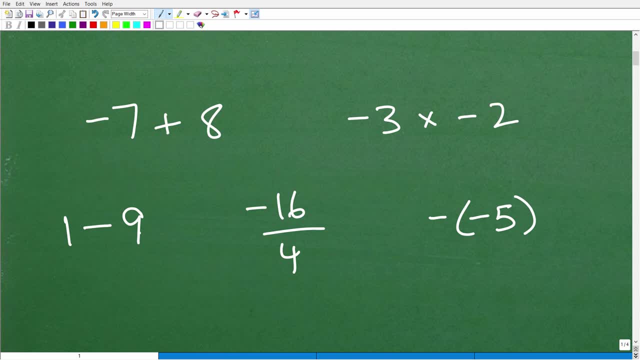 we're talking about. And, again, these are not that difficult to do, but they're easy to make a mistake, because students, you know, stop and they go. I kind of forget the rules. What is it? again, You know, they kind of know it. But if 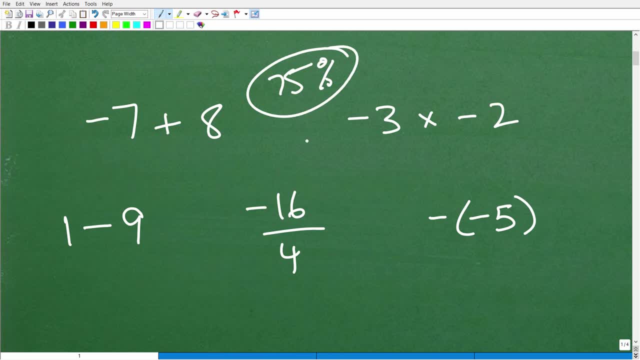 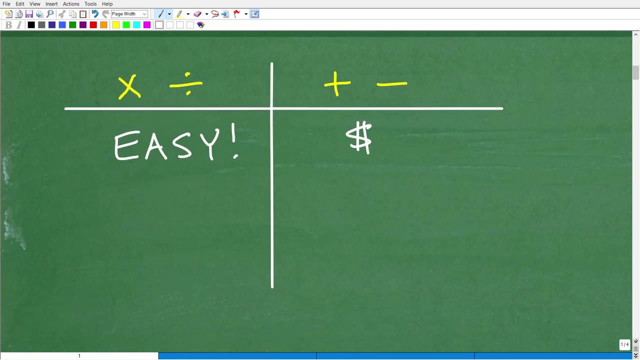 you're 75%, you know, remember these rules. Well, that doesn't being close isn't going to cut it, because it's. you have to know these rules and remember what you're doing 100% of the time. But let's get into this stuff, And I want you to think of positive, negative numbers as being just two. 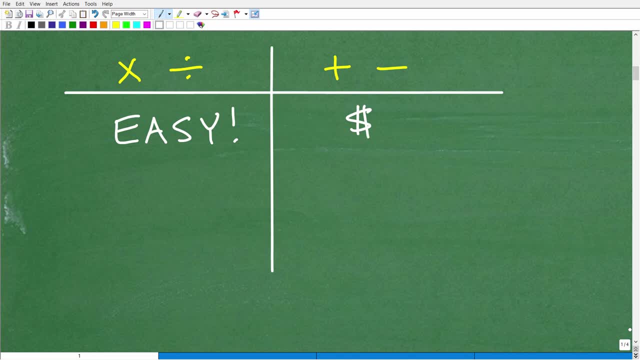 rules, two rules and two rules only, And let's break this up. So the first rule is going to be what we do with multiplication and division, And then our second rule is for addition and subtraction, And let me go ahead and just break this down this way. This is easy. So for 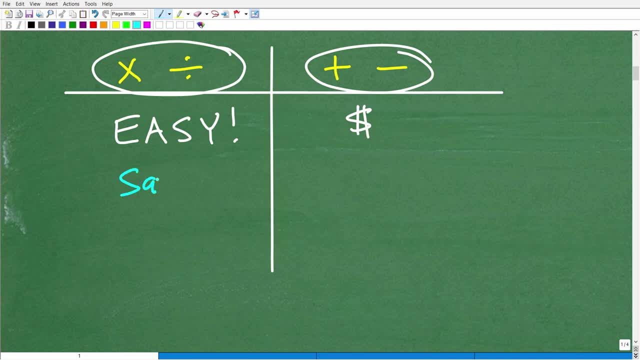 multiplication and division. it's easy because it's the same rule. It's the same rule And it's like the easiest rule ever I'm going to show here in a second, And then here you can see I have something about money when it comes to addition and subtraction, And then I'm going to show you how to do that. So 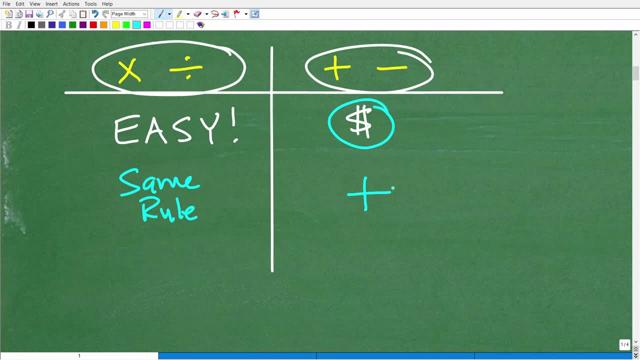 typically I want you to just to think: if you know how to add, then you're going to know how to subtract, Okay. so I want you to kind of group mentally what's going on. So multiplication, division, it's super easy, It's the same rule And anytime you see addition and subtraction, 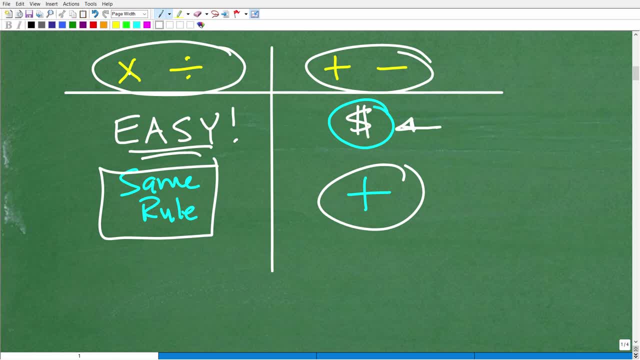 it's basically just going to be the addition rule, And we want to think money. Okay, so this is good. I mean, we're talking about things that we like. we like things that are easy and we like money, So we're on the right track here. All right, let's go ahead and talk. 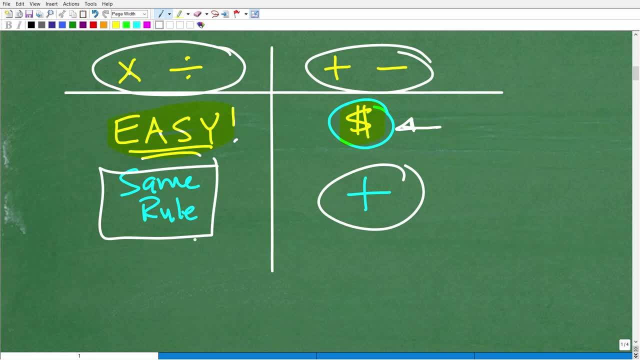 about multiplication and division, And we'll take care of 50% of the rules. right, Because we're talking about adding, subtracting, multiplying and dividing. right here, we're going to take care of this rule, the two out of four, these rules right now. Okay, so what's the deal? Well, 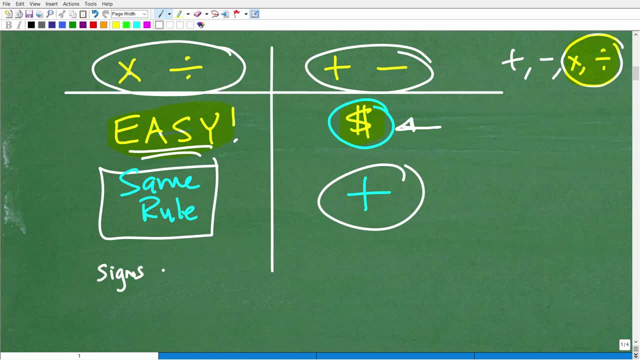 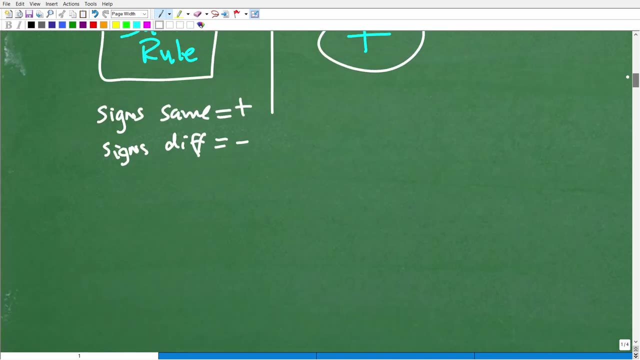 if the signs are the same, okay, if the signs are the same, the answer is positive. If the signs are different, this answer is. answer is negative, Okay, it's. it's so, so easy. Let me go ahead and show you again. we're talking about multiplication and division. So negative, three times negative. 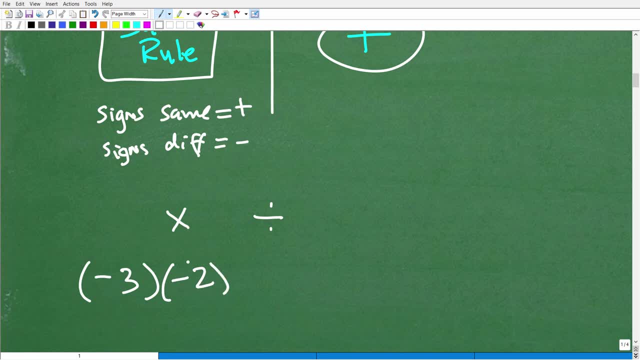 two. Okay, so we can write that this way: negative three times negative two. What do we have? Do we have the same signs? Yes, we do. They're both negative. Okay, so our answer is positive. So we're just going to multiply three times two is six. the answer is positive. That it's. 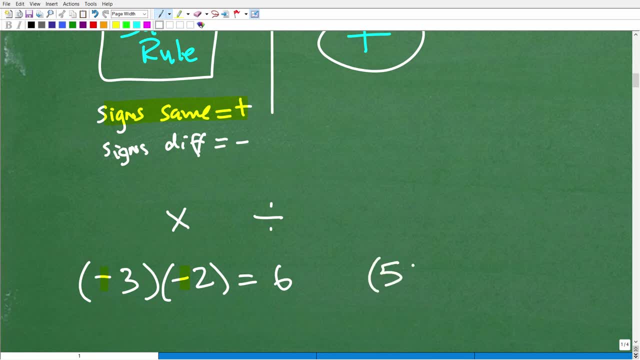 it's as simple as that. Let's go ahead and just change this up. How about a positive five times a negative three? Okay, well, what's the situation? Remember you, focus in on the signs. the signs are different. I got a positive here and a negative here, So I'm just going to multiply. 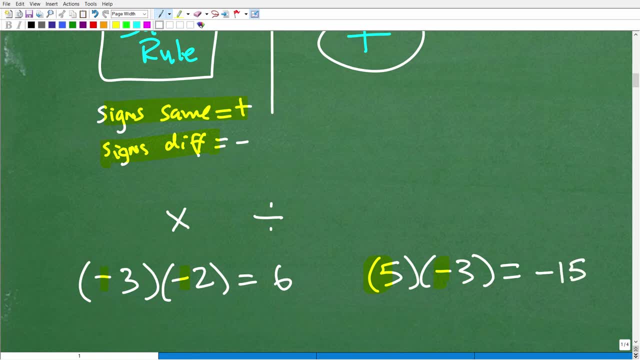 and the answer is going to be negative. Okay, it's as simple as that. Five times three. I'm just considering what the sign is. Oh, this one's positive, this one's negative. it's different signs, So it's always going to be negative. I mean, we don't need to make it that. 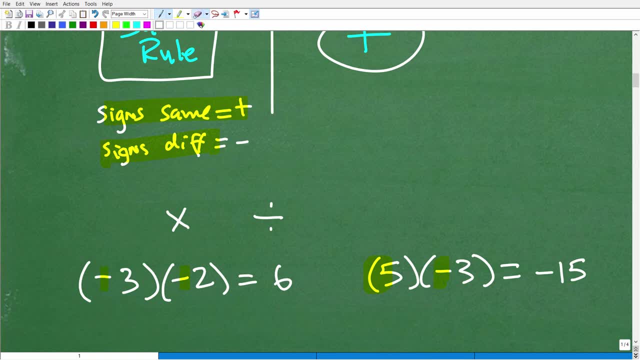 much More difficult than what it is. It's a very basic rule And it's the same rule for division. So let me show you this now. What if I had negative 25 divided by negative five? Okay, well, what are? 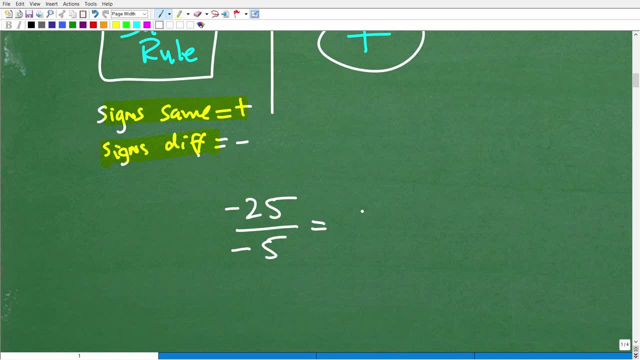 the signs. Are the signs the same? Yes, they are negative, negative. So the answer is 25 divided by five, which of course is a five, and it's going to be positive. How about a 14 divided by negative seven? Okay, well. 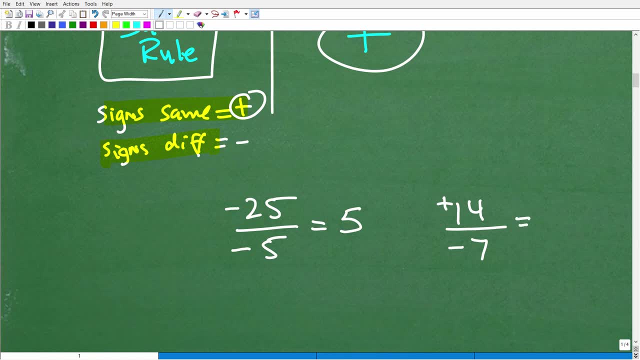 signs are different. This one is positive, this one's negative. So our answer is negative, So this will be a negative two, All right. So again, I wasn't lying to you when I was telling you this is super easy And already right off the bat. okay, you already got 50% of these operations down. 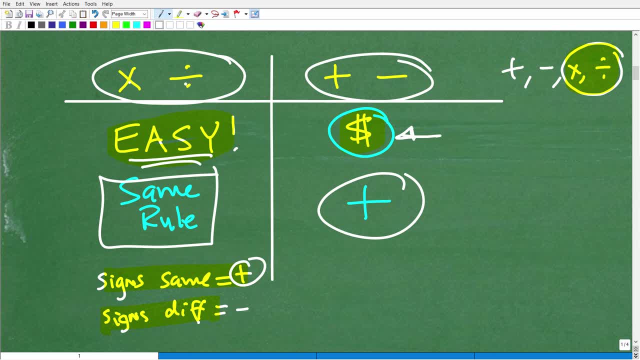 So don't confuse multiplication and division. Okay, it's the same sign And it's super easy. So now let's get into adding and subtracting, And really we're talking about just an addition rule. we want to talk about money. Okay, because we want to model something here, And money is a great 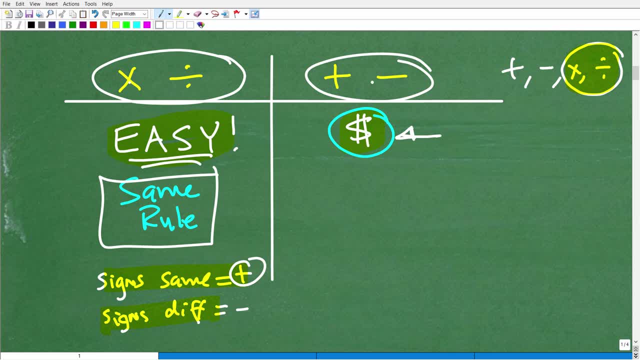 money. situations are a great way to model positive and negative numbers when we're adding and subtracting them, So I'm going to show you exactly what I'm talking about right now. Okay, So let me ask you this question: Would you rather have $100, $0, or negative $100?? Okay, 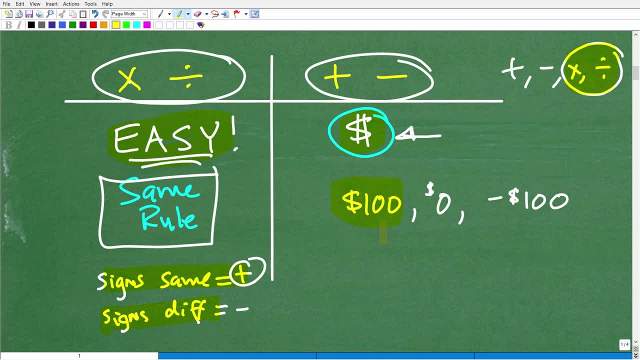 All right. So most of you out there are going to say: I'll take the 100 bucks. That's the most money here. But what about between zero and negative 100? What would you? what would your situation? What would you rather have in terms of your financial situation? Hopefully you said zero, I'd rather. 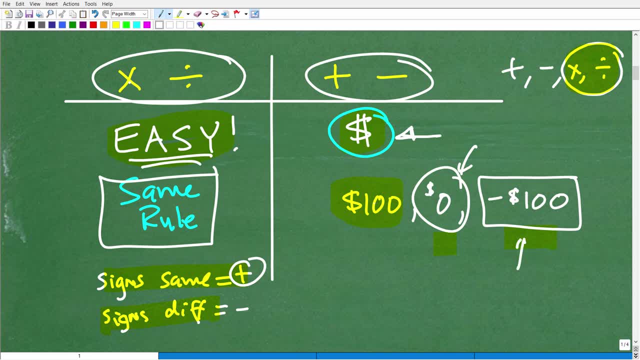 have $0 and negative $100. What does this mean? What does negative $100 mean? Well, it means that you have less than $0.. This is debt, right? Let's kind of look at it this way here. Let's talk about. 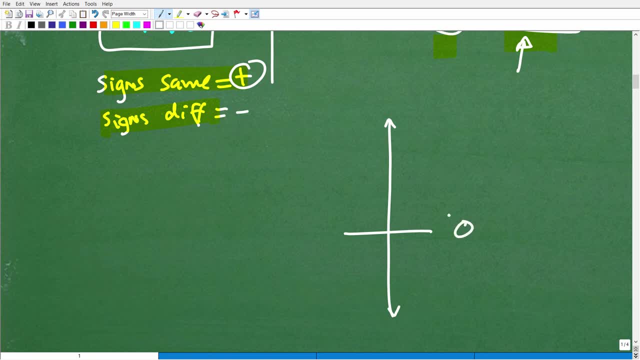 money respect this way. Okay, so let's say I have zero bucks right there And up here I have $100.. That's great. So here I have money or here I have no money. But then I start having actual money. 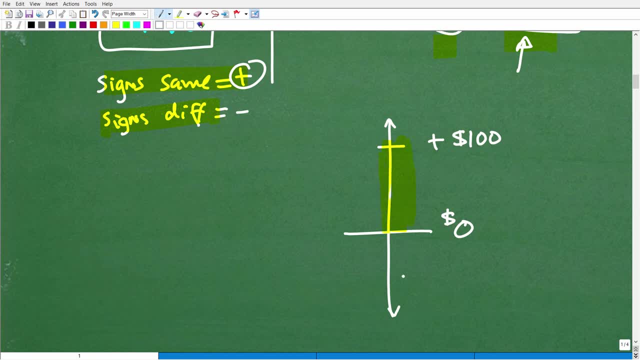 that I can use Now. But can we go the other way? Yes, you can. Unfortunately, you can go down here and have less than no money. Okay, you can have debt. Yeah, So anytime you see a negative sign associated with money. 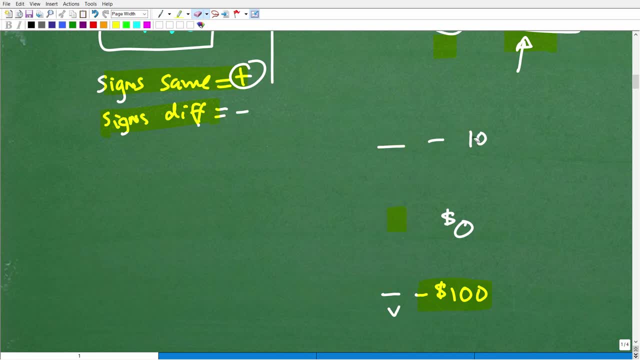 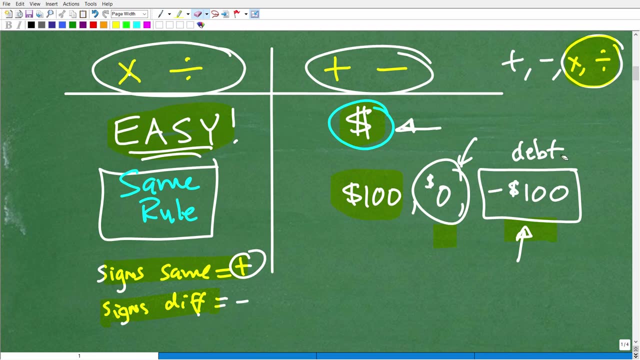 that's debt. Okay, so it's actually less than zero. Okay, that's what we use- positive and negative numbers- to express things like money and debt and whatnot. they come in very handy, All right. so let's take a look at a problem here. Let's start off with something like this. Let's say: you have 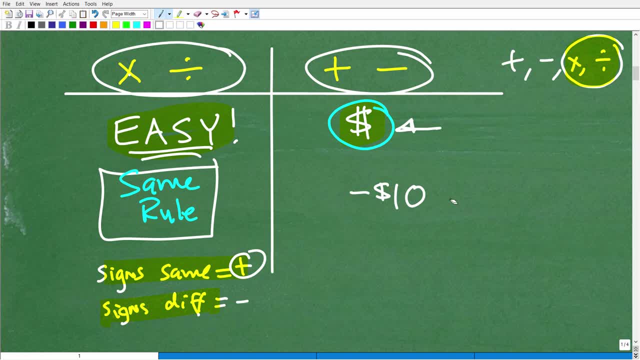 a you have, let's, let's. let's do it this way. Let's start off with negative 10 plus seven. All right, negative 10 plus seven. let's think of this as debt, something that you owe, So maybe you. 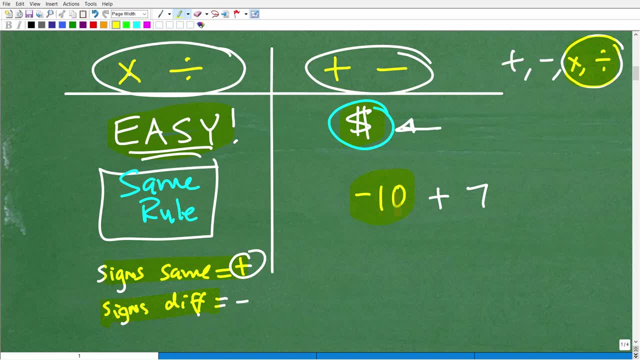 borrow 10 bucks from your, your your best friend. you borrow $10 from your best friend And now your best friend comes up to you and says: Hey, I want my money back. give me that negative $10 that you gave back to me. But you actually have $7 in your pocket right now. You're like: I got $7 in your 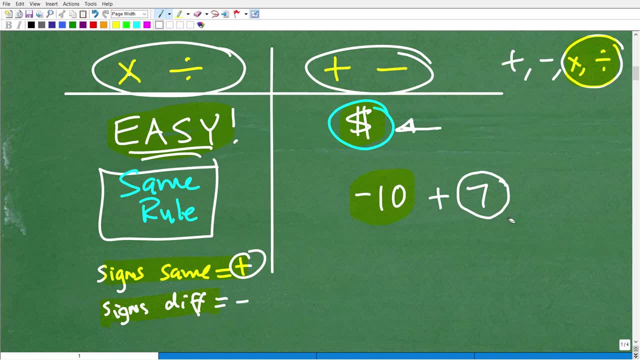 pocket. So if you gave your friend- you gave your best friend- $7, you're like: I got $7 in your pocket. What would be what? do you still owe them? Okay? Well, if you owe your friend $10, but you have $7 to 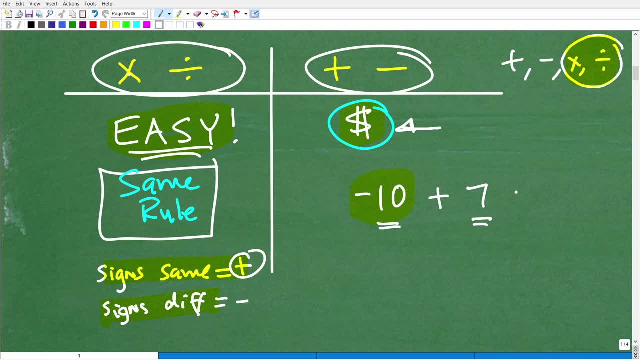 pay them back. how much do you still owe your friend? Okay, hopefully, you're seeing that it's going to be $3.. Okay, you're still going to owe your friend $3.. So, when you're looking at positive and negative numbers that you have right here, you have more debt than you have money. Okay, So if 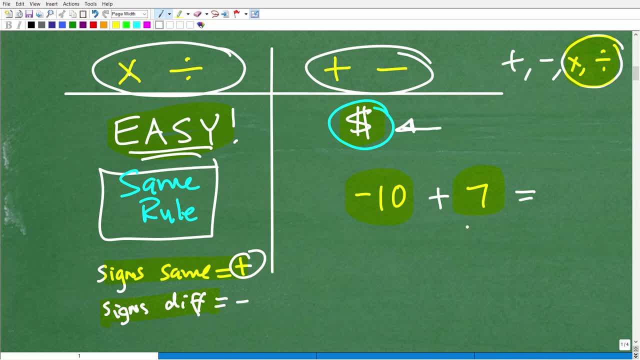 your friend says: Hey, give me my 10 bucks. So I don't have 10 bucks, I don't have 10 bucks, I don't have 10 dollars. I'll give you my $7 and I'll owe you $3.. Okay, So here is what happens when you're. 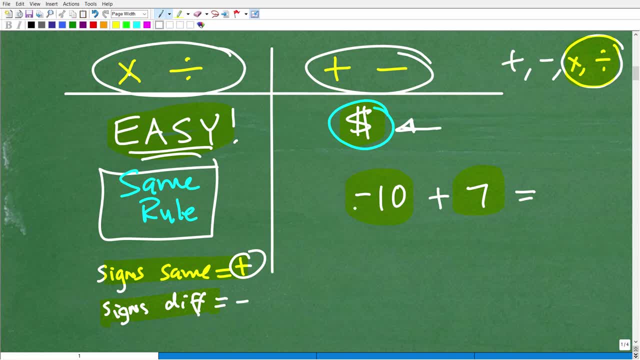 adding positive and negative numbers. Okay, when one is positive, one's negative. you're always going to subtract the two. Now we just have to determine what sign it's going to be. Okay, well, in this case, you have more debt, more negative numbers. okay, then you do positive. So we still. 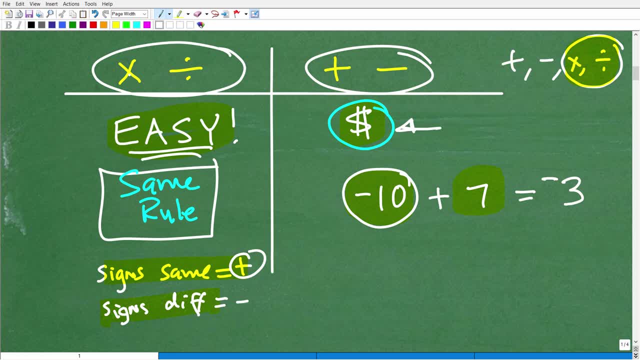 owe your friend $3.. Okay, so that's kind of the way you want to think. That's why I like to use money as an example. Let's go ahead and do another example. What about this? Let's say you have $12 and you owe someone $8.. Okay, so 12 plus negative eight. Okay, so what? 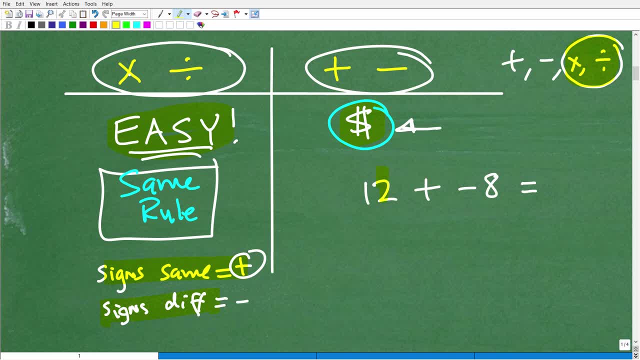 is 12 plus negative eight. All right, so you have 12 bucks in your pocket. your friend comes up to you and says: Hey, can you give me my $8 back? All right, because you owe right. this is like debt. 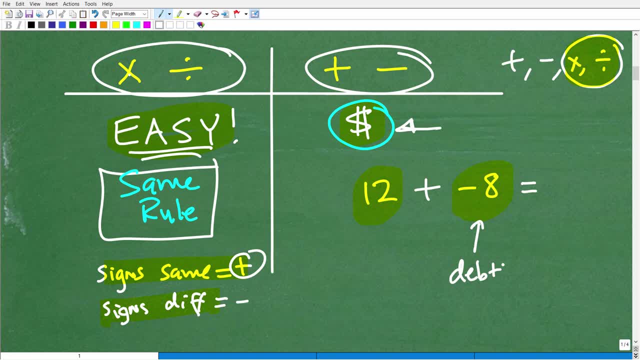 you owe, or you just got a bill for $8.. How much money do you really have? Well, you have 12.. Now you're going to pay your bill, you're going to pay off your debt. that's negative eight, so you're left with positive four. Okay, so 12 plus. 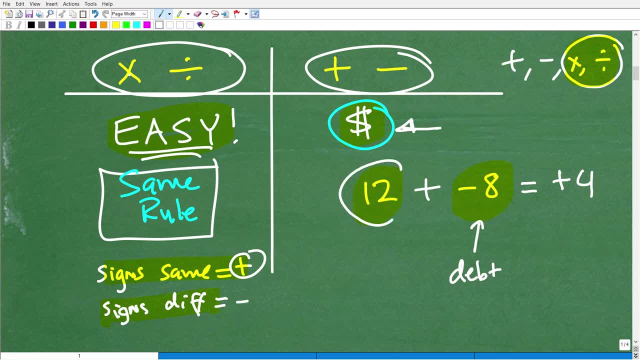 negative eight. again, you subtract the difference, But this is the larger number. it's positive four. So you don't want to remember these things. in terms of a rule, I like to use money as a good model, So it just kind of makes sense. right? You have 12 bucks, you owe someone or you just got a. 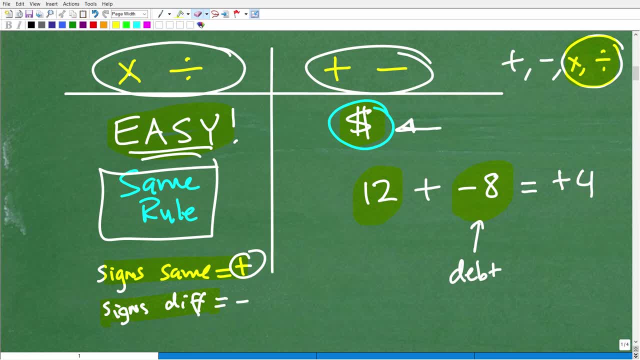 bill for $8, you pay that off, So you still have positive $4.. Okay, that's as simple as that. Now let's go ahead and take a look at some more examples. What if you have negative two plus negative three? So last week you brought two bucks from your friend. This week you 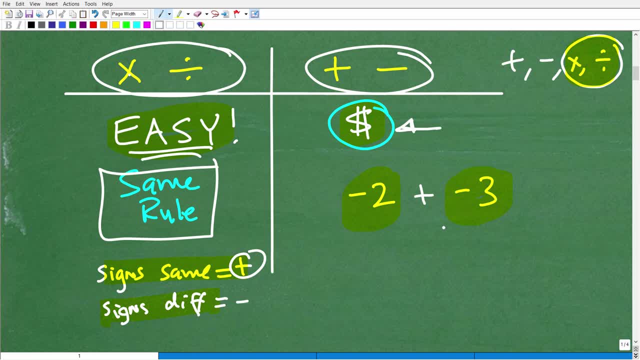 borrow $3 from your friend, And so how much collectively do you owe your friend? Okay, well, negative two plus negative three, you have a total of $5 in debt. Okay, so that's how you would handle that situation. So, negative two plus negative three, you have a total of $5 in debt. Again, use this money example. 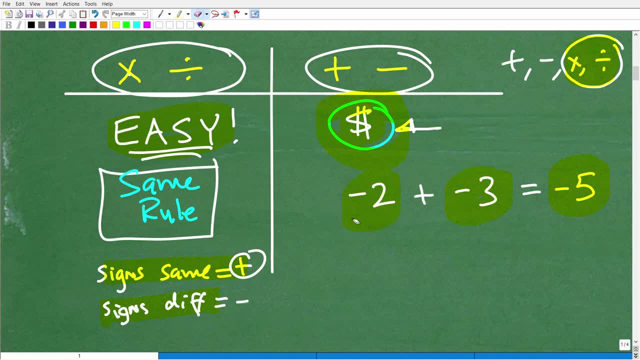 All right, All right, Now. we've done everything here except talk about subtraction. So let's talk about subtraction. And I basically said that you're going to just remember one rule, and that's for addition. So I just showed you how to add positive and negative numbers. Remember you just? 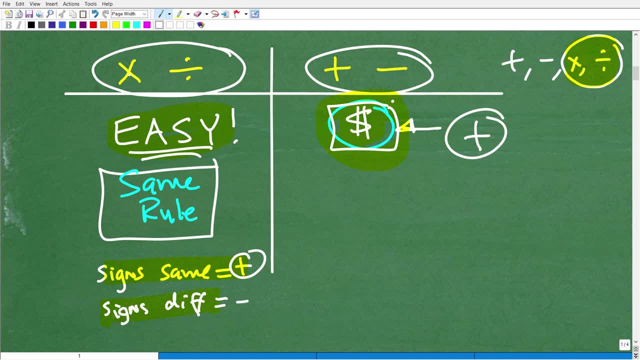 want to use common sense and think of the signs of those numbers as either you having money or having money, Okay, and just kind of stop and slow down And you can kind of figure this out. But let's take an example like this: three minus seven. Okay, so we've got three minus seven. Well, a great way to 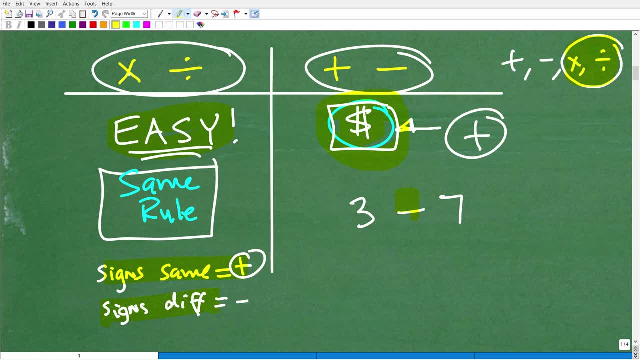 subtract positive and negative numbers is to change the subtraction sign into an addition sign. So we're going to rewrite this problem like this: three plus. Now when we do this, when we change a subtraction sign into an addition sign, what we're going to do is something called plus negative. 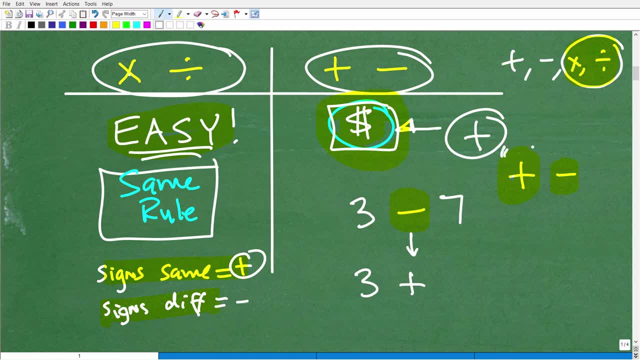 I'll say that again. It's called plus negative. I'll say it one more time: Plus negative. So what we're going to do is we're going to change that subtraction sign into an addition sign. We're going to do plus negative, So we're going to do change this into an addition. We're going to put a. 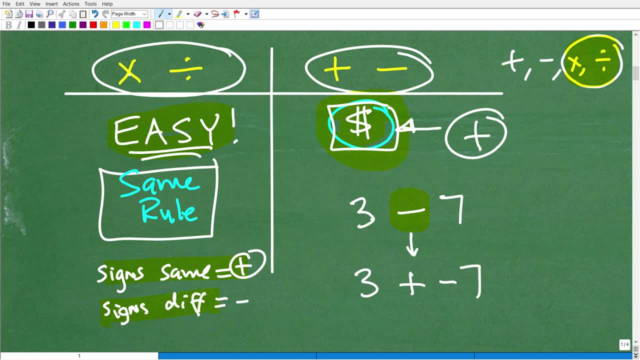 negative to the right of that, And then we're going to put our number right there. So we have three minus seven. So we're going to do plus negative. So now we have three plus negative seven. Okay, so now we're back to an addition problem. So we have three. 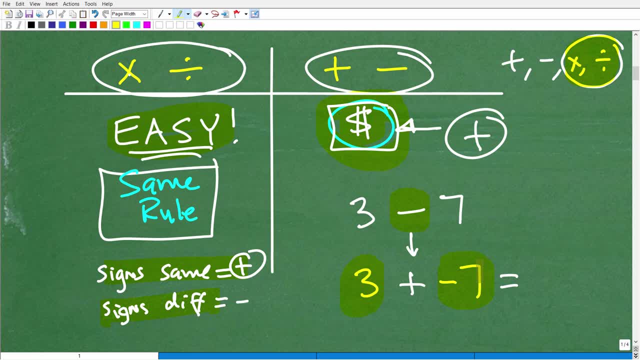 But now we our friend comes up saying: hey, give me my $7 that I lent you last week. You're saying: well, I can only give you $3, but I'll owe you $4,, right, So three plus negative seven. 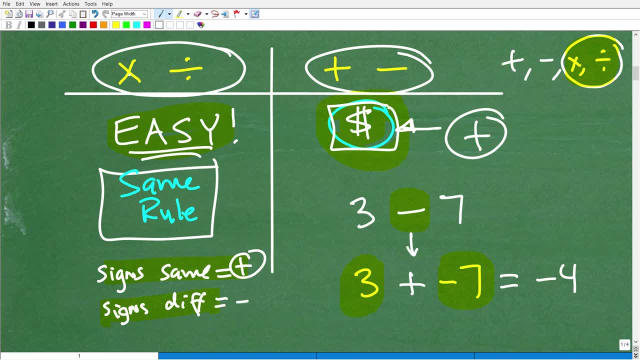 is negative four. Okay, so that's how we deal with subtraction problems. Now let's take a look at a couple more examples. What if I had negative three minus seven? Okay, well, we're going to go ahead and do our plus negative again. So this would be minus three plus negative. 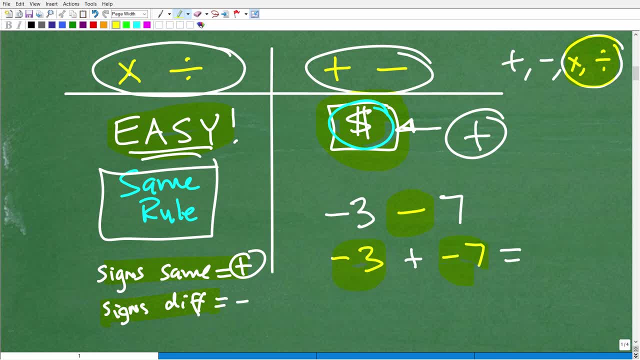 seven. So now I have $3 in debt and $7 in debt, So we're going to have a total of $10 in debt. Okay, so now there's one other quick situation. Let's go ahead and talk about it now. What if I? 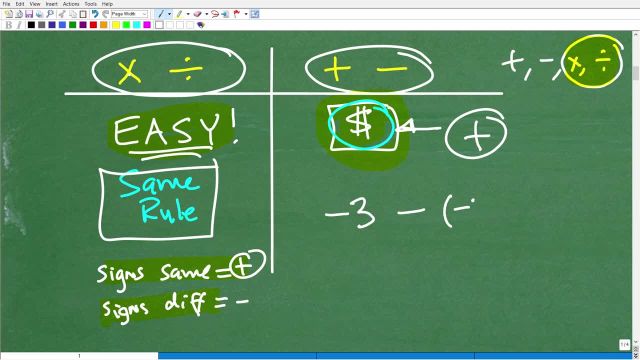 had minus three minus a minus two. All right, negative three minus a minus two. What about this scenario? Well, we want to discuss real quick what a negative of a negative number is right. So like negative of a negative two. This sign in math, this negative. 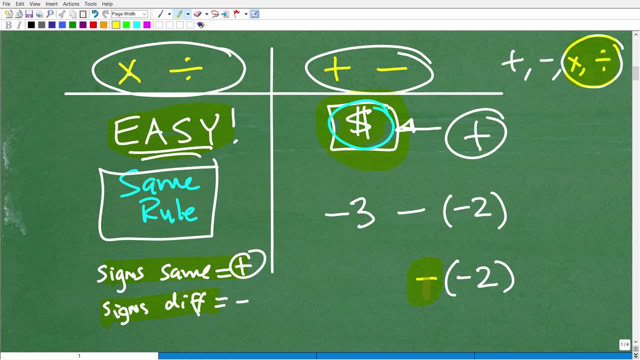 sign. oftentimes we can think of this as the opposite sign. So this is like the opposite of a negative, two or a negative times a negative. Remember, the signs are the same. So a negative of a negative or a negative times a negative, or the opposite of a negative, it's positive, Okay. 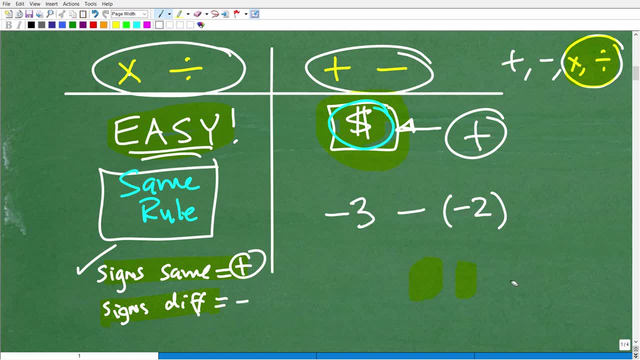 so a negative of a negative is positive. right, We just want to remember that. So what do we have? minus a, minus two. Okay, we can think of this as plus negative, or plus a negative of a negative two. So this is going to be negative three plus a negative of a negative two. Again, it's positive.